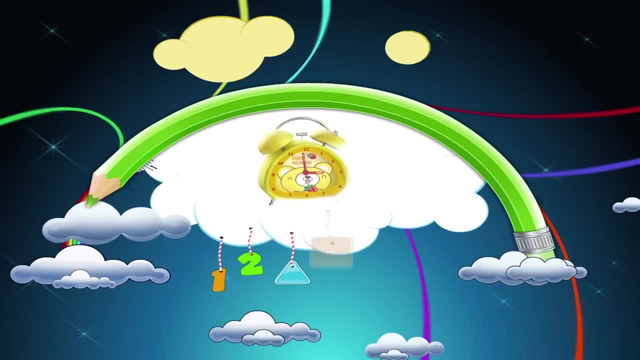 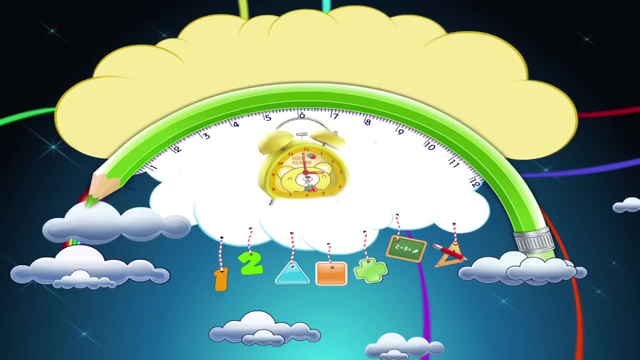 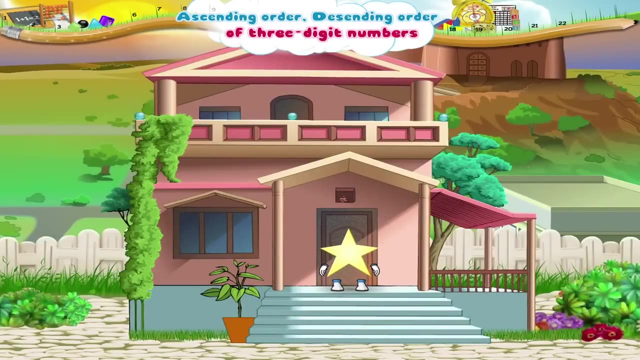 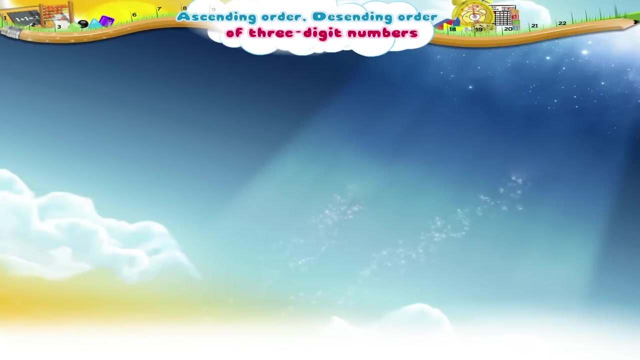 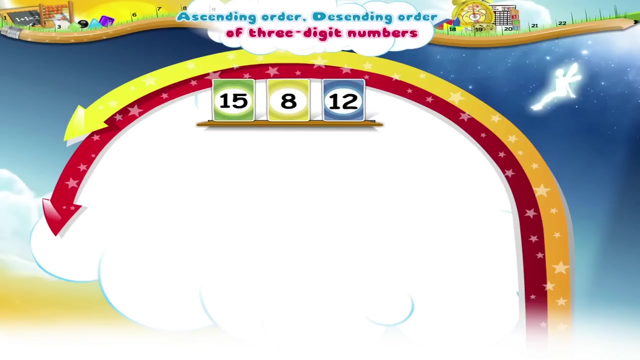 Ascending order. Descending order of three-digit numbers. Starry, why are you running up and down the stairs? Oh, for fun. Hmm, let's have some more fun. Here are some stickers with numbers. Put them on the steps in the ascending order, that is, from the smallest to the biggest. 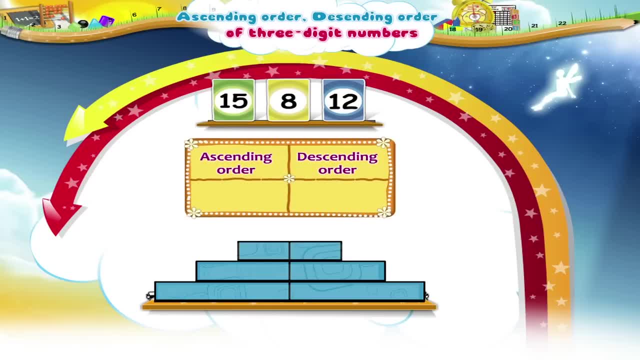 Very good. So now tell me how many numbers are there in the ascending order? Tell me the ascending order of these numbers. The ascending order is 8,, 12 and 15.. Now tell me the descending order, that is, from the biggest to the smallest number. 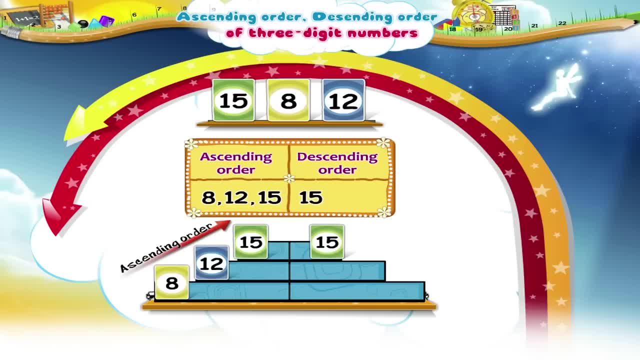 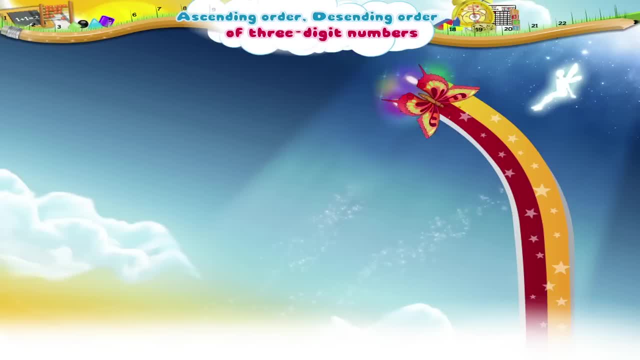 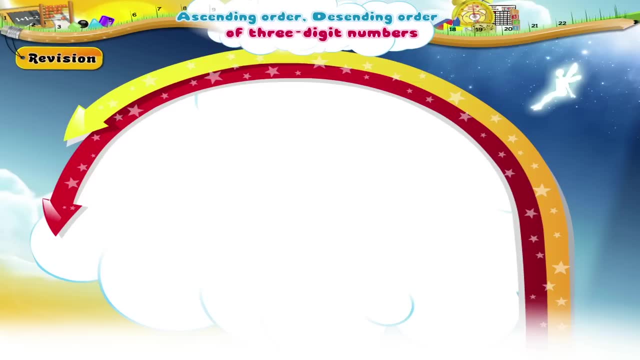 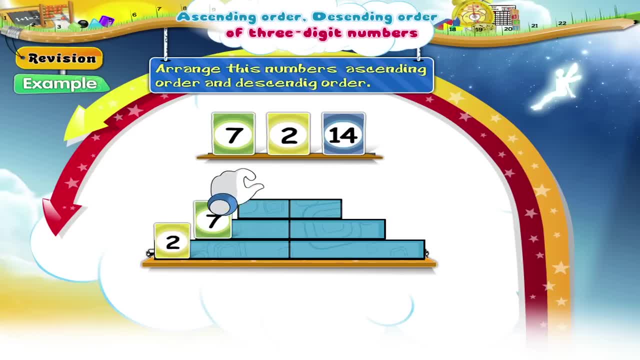 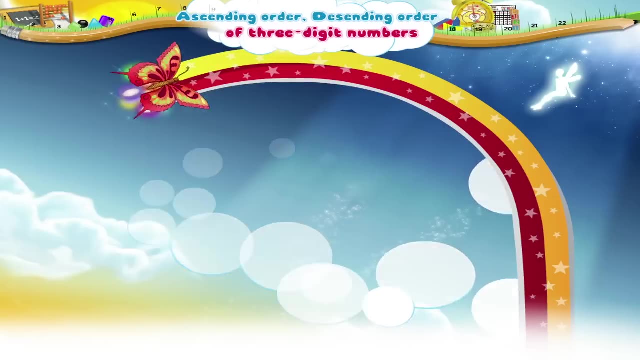 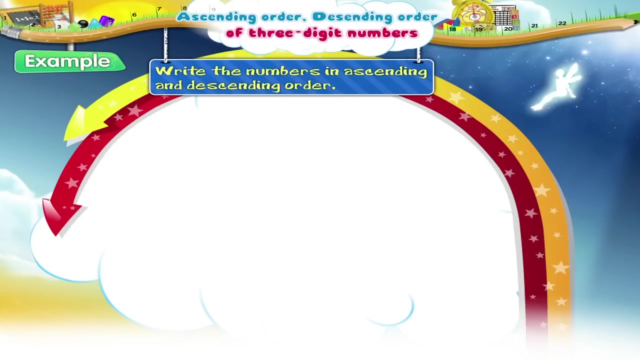 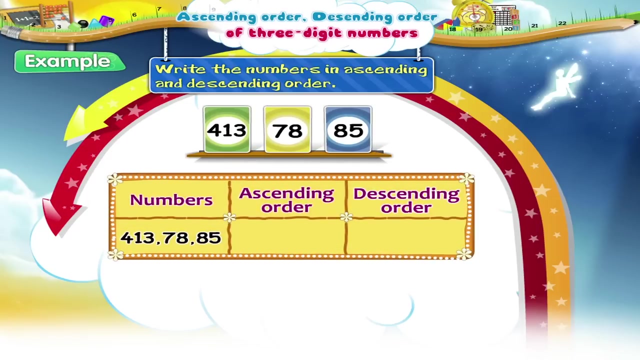 Here, take some more stickers. Here. take some more stickers. Now write the ascending order and the descending order. The ascending order is 78,, 85 and 413.. The descending order is 413,, 85 and 78.. You are very smart, Sturry. 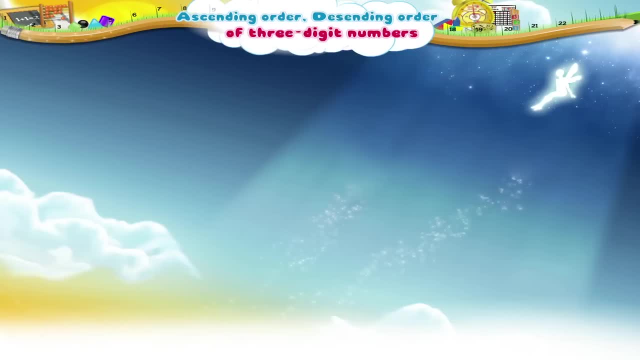 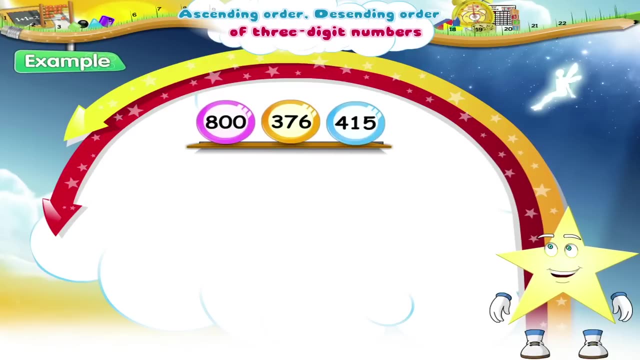 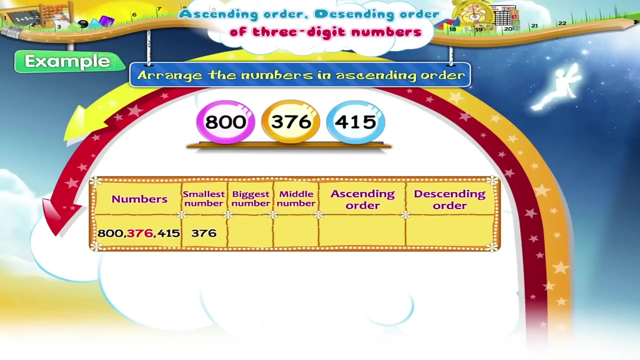 Sturry, look at these numbered balls. Arrange them in the ascending order of numbers. What happened, Sturry? You seem to need some help. Okay, let's do it together Here. the smallest number, The smallest number is 376 and the biggest number is 800. 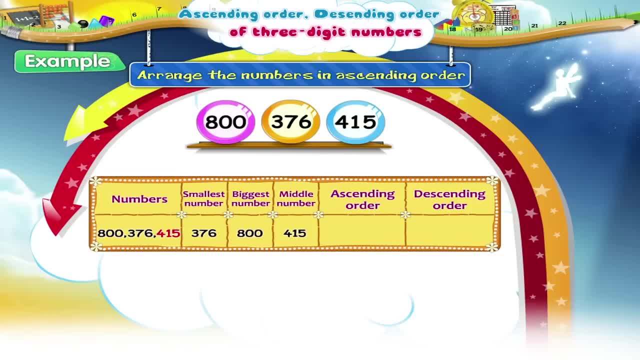 So the middle number is 415.. So the ascending order will be 376, 415 and 800.. Now for the descending order. we will arrange the numbers starting from the biggest number. So the descending order is 800, 415 and 376. 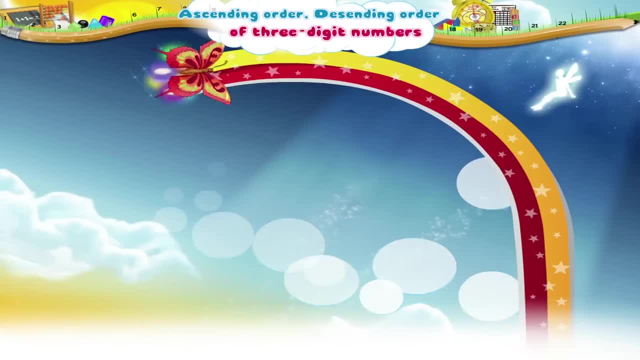 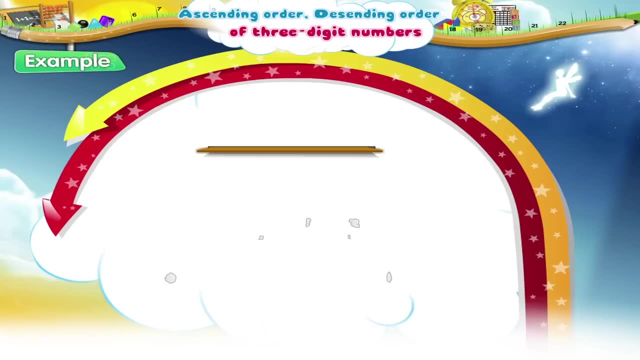 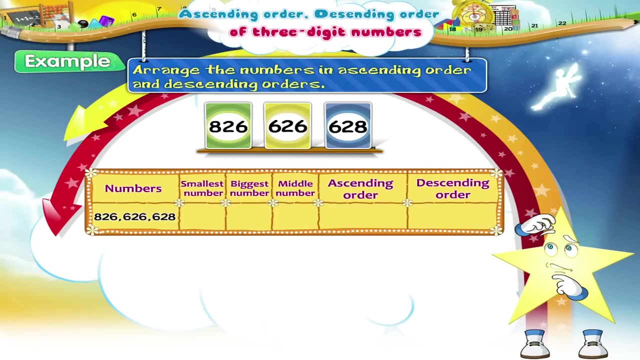 Now, let's do it together. Now take these stickers and let's arrange them in the ascending and descending order of the numbers shown on them. Starry, which is the smallest number here? Good, it is six hundred and twenty-six. 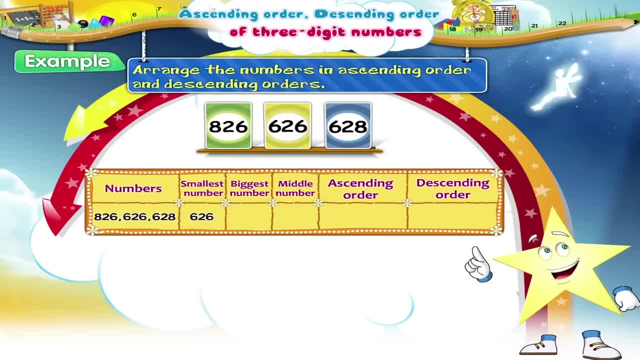 And which is the biggest number. Right, eight hundred and twenty-six is the biggest number, So the middle number is six hundred and twenty-eight. Now place the stickers in the ascending order and the descending order, Starting from the smallest number. The ascending order will be the smallest number. 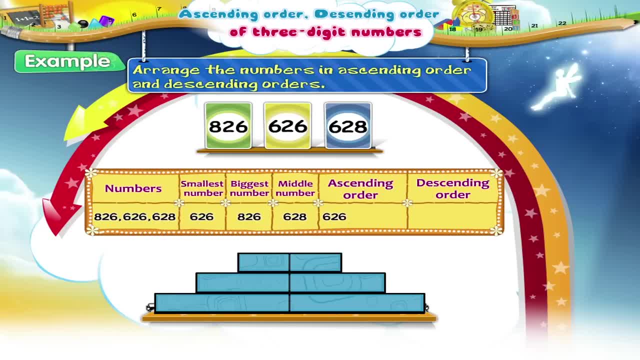 The descending order will be six hundred and twenty-six, six hundred and twenty-eight and eight hundred and twenty-six. Starting from the biggest number, the descending order will be eight hundred and twenty-six, six hundred and twenty-eight and six hundred and twenty-six. 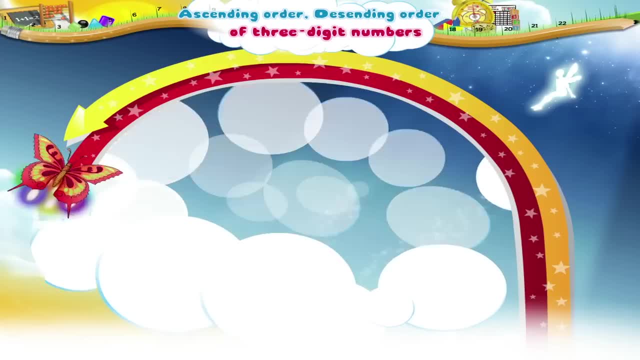 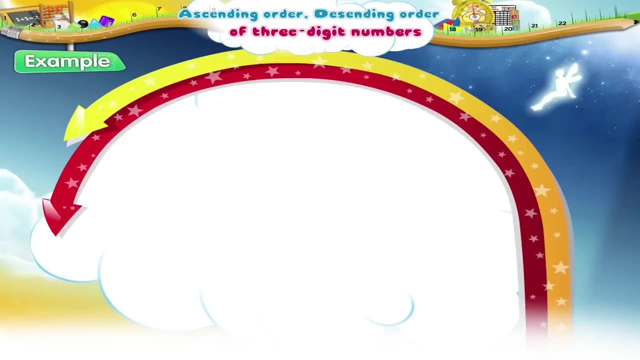 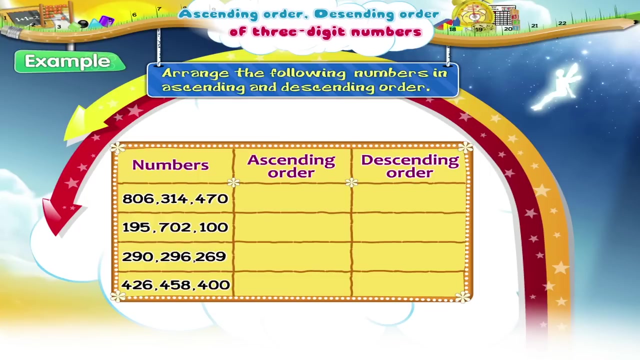 Good job, Starry. Let us revise what we have learnt. Arrange the following numbers in the ascending and descending order. For the first set of numbers, the ascending order is 314,, 470 and 806.. And the descending order is 806, 470 and 314. 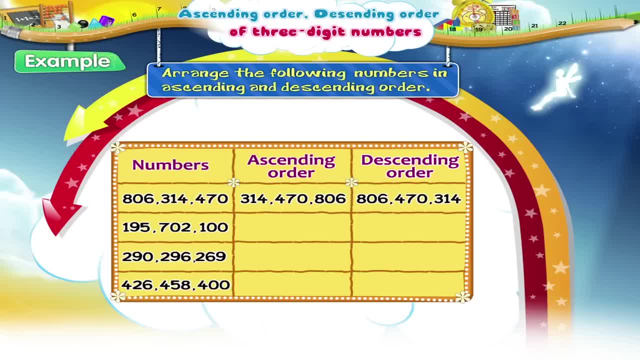 For the second set of numbers, the ascending order is 100,, 114,, 195 and 702.. And the descending order is 702,, 195 and 100.. For the third set of numbers, the ascending order is 206,.